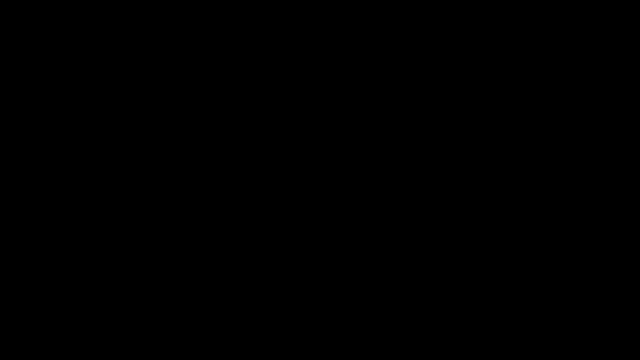 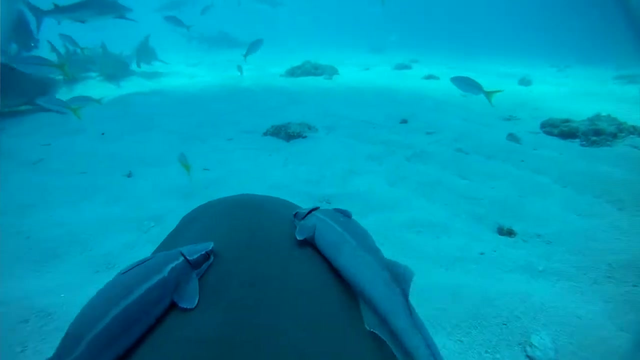 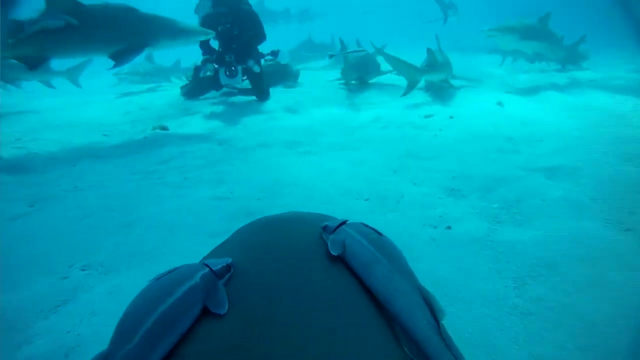 of sharks could have ecological consequences. There's been a surge of recent studies that have tried to try to understand this question about how human shark diving impacts the behaviors of sharks. However, over relatively smaller time scales, this is the first study published to use satellite. 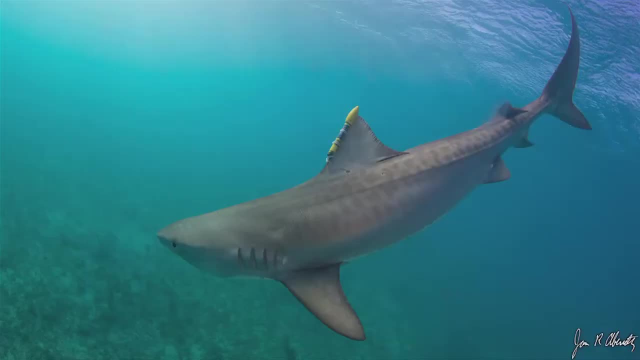 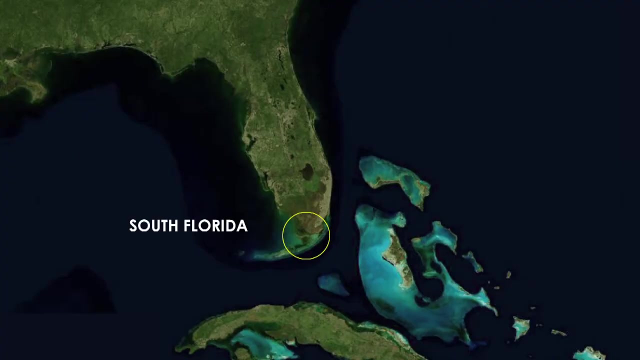 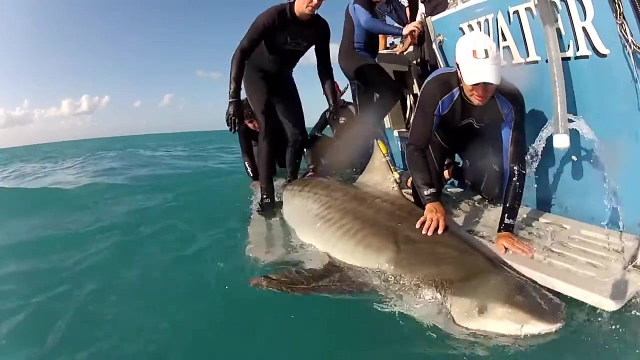 telemetry to explicitly look at the impacts of shark diving on tiger shark long-range movements. In Florida, shark diving using bait is illegal And in the Bahamas it's highly practiced. So we went to these two spots. We satellite tagged a bunch of tiger. 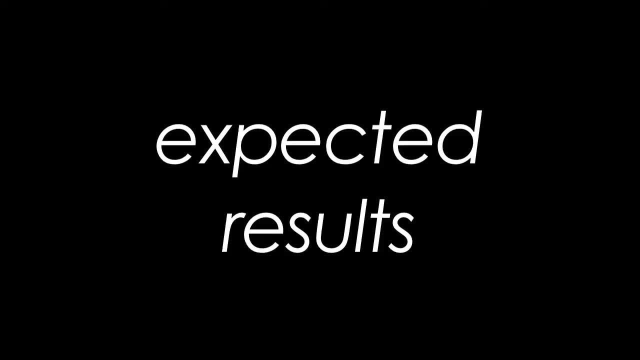 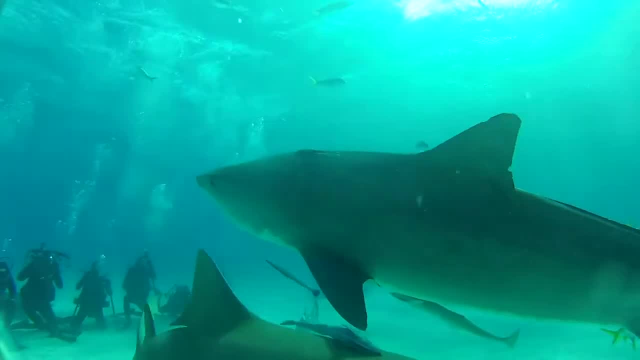 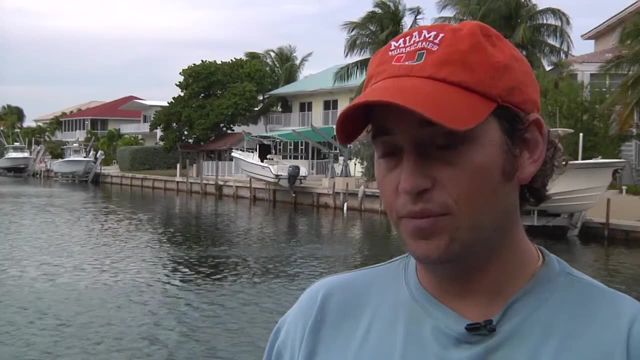 sharks in each location and looked to see how they moved. So we expected that at Tiger Beach, at the ecotourism location where they're being fed, that those sharks would show more restricted movement and an activity space that kind of centered around that spot. In comparison, we thought that sharks tagged in Florida would. 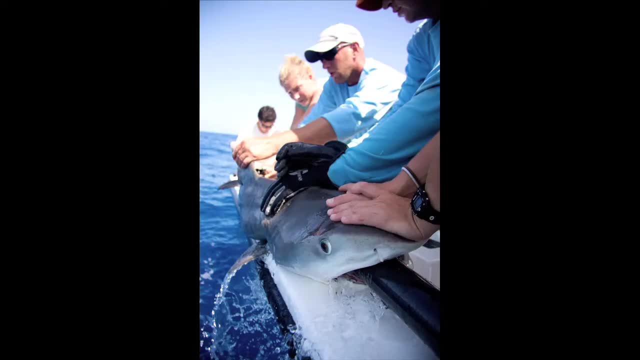 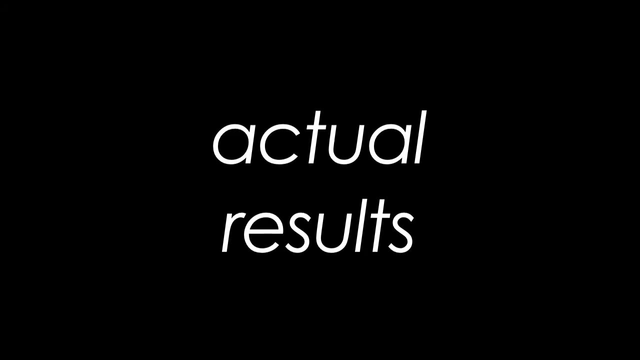 have a relatively larger dispersal and show less sight-attached movements than the sharks tagged in the Bahamas. But what we found was exciting and not what we expected. We found that the sharks' movement was more restricted than the sharks' movement in the Bahamas And we found that the sharks' 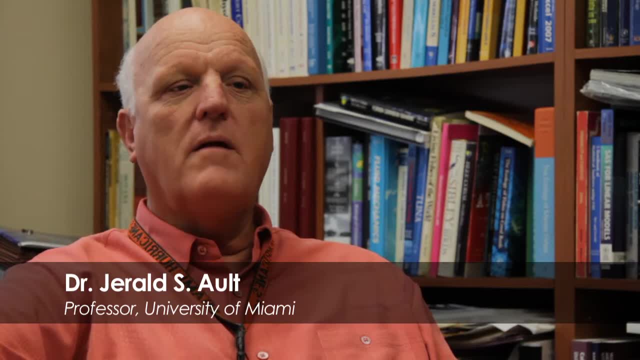 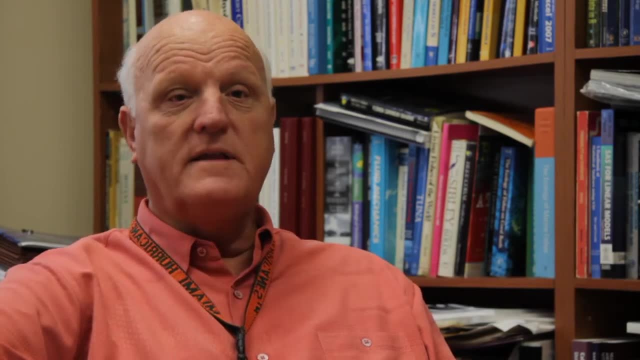 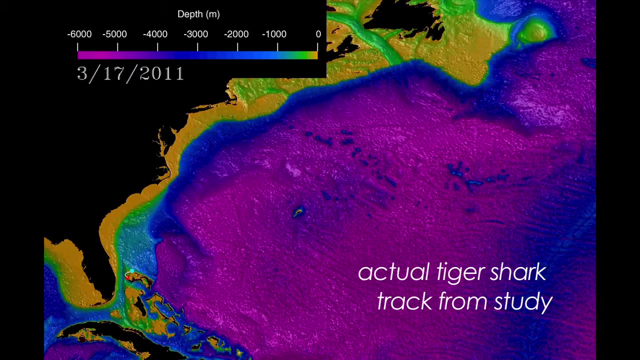 tag in Florida was less restricted than the sharks' tag in the Bahamas, But what we found was exciting and not what we expected. Some of those sharks quickly moved over 3,000 kilometers away and spent months at sea. The Florida sharks showed behaviors that are very similar to the tiger sharks from Tiger Beach, So they both made these. 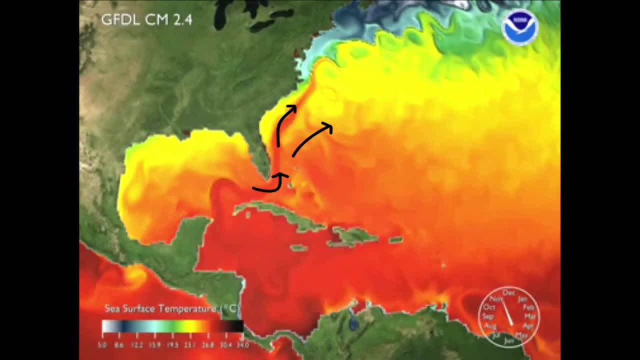 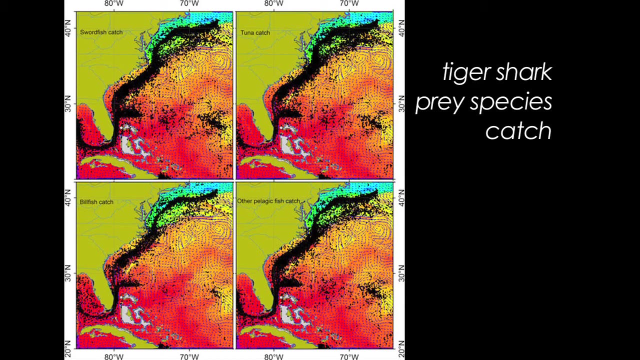 long-range movements with their pedigrees that they had to make to keep their eggs from long-distance migration patterns following the Gulf Stream to areas of the Atlantic that have high productivity. The Gulf Stream served as a pre-aggregating device for these large tiger sharks that go. 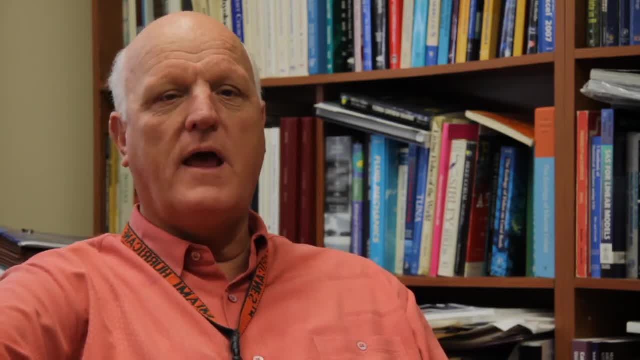 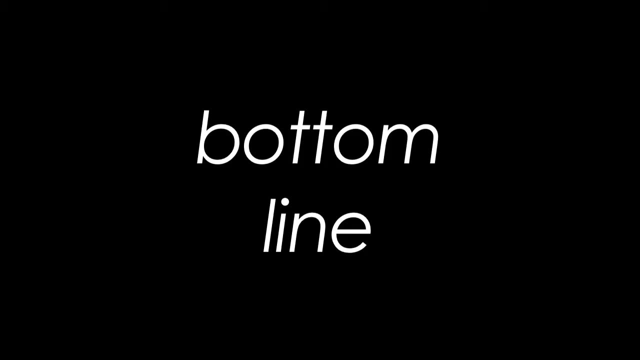 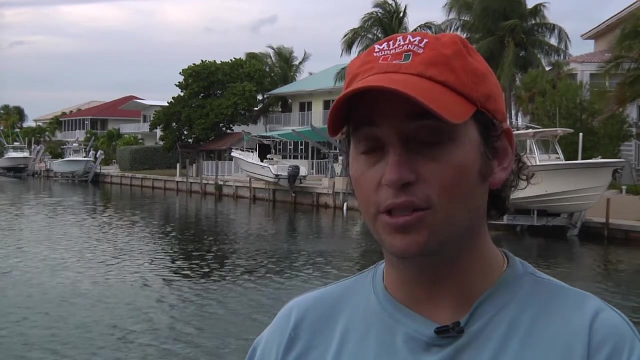 out on feeding forays, basically one to build up the gonad and to service the juveniles before they go back and pup the animals to the south. I think the take-home message of this study is that, rather than rushing to make conclusions,